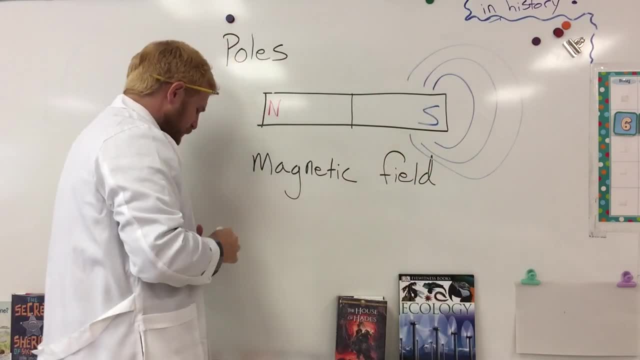 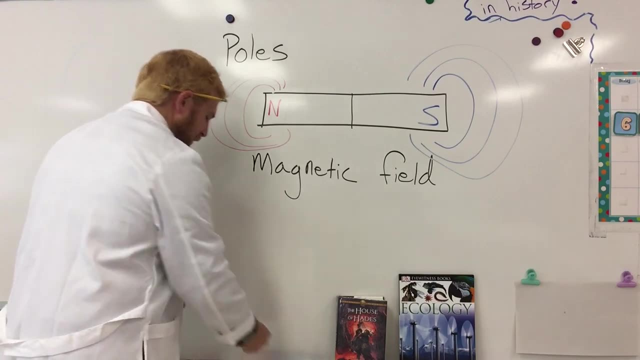 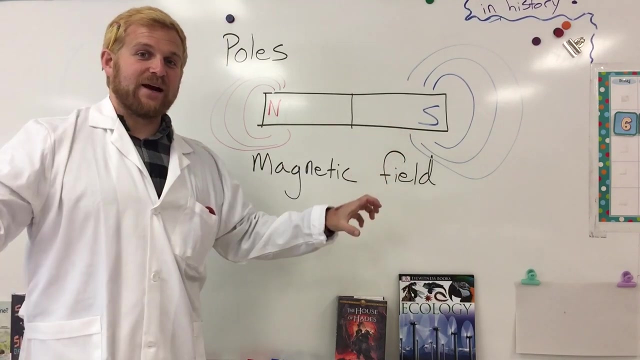 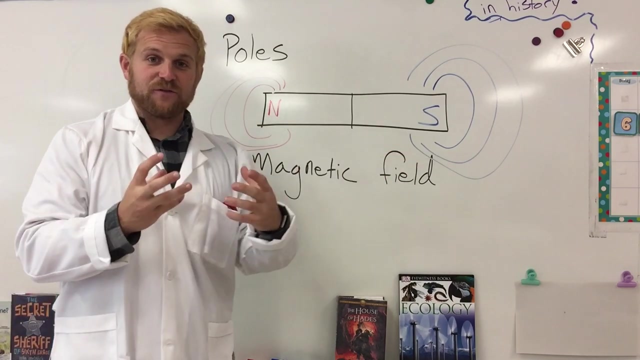 field, just like this here, And the north sends out a north field. Now what does that mean for our magnets? It means that the north field and the south field are both reaching out for the other field. So our north field is looking for some south field to attract to and our south field is looking for a north. 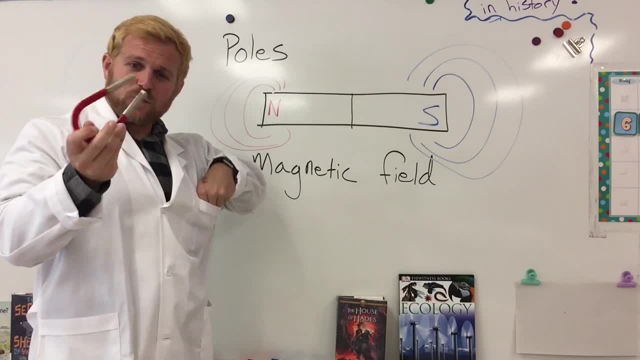 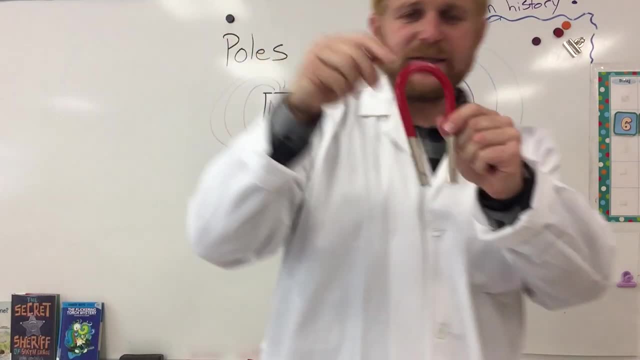 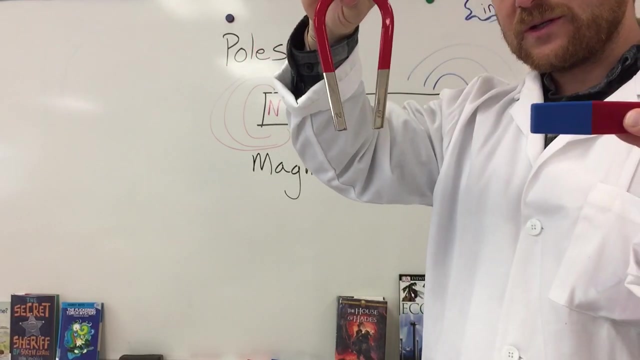 field. This can be demonstrated with a horseshoe magnet and a bar magnet. Here's my horseshoe magnet and you can see it's labeled with a north pole and a south pole. Now, this one is not labeled, but we know that our north pole wants to be attracted to the south pole of 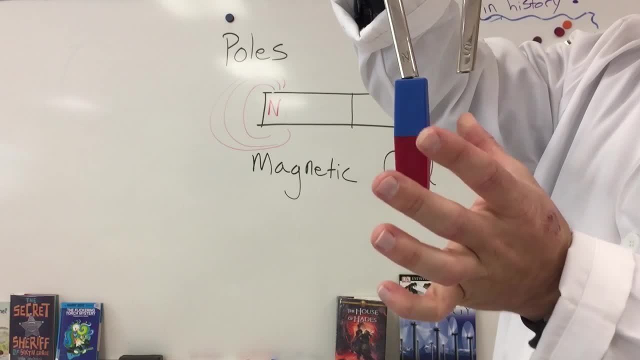 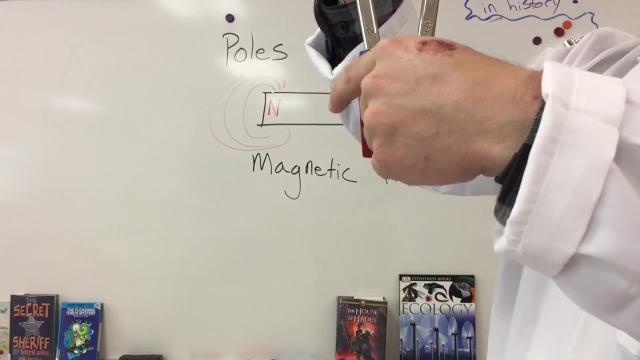 this bar magnet. So let's find out, Let's put this here and look. it's attracted to it, So we can assume that this is the south pole of the bar magnet If I flip it over and try and do a north. 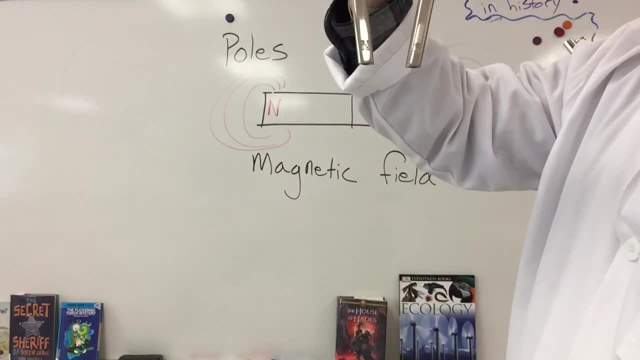 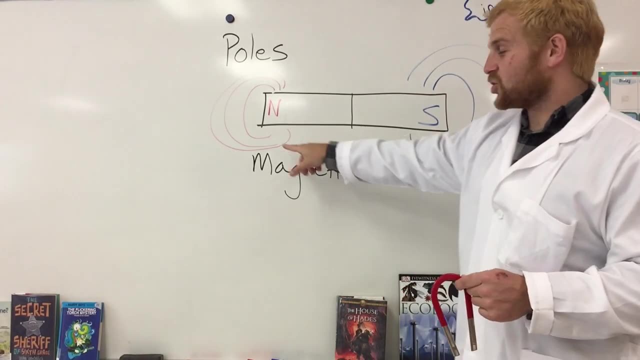 pole to a north pole, it's going to be attracted to the south pole of the bar magnet. So we can see that the north pole it won't hang on because the north pole is attracted to the south pole and the south pole is attracted to the north pole With some magnets. this magnetic field is so strong. 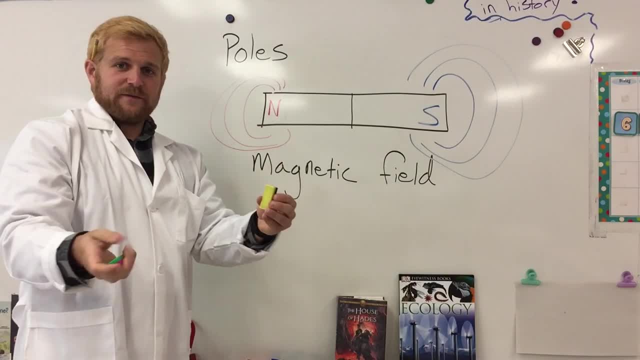 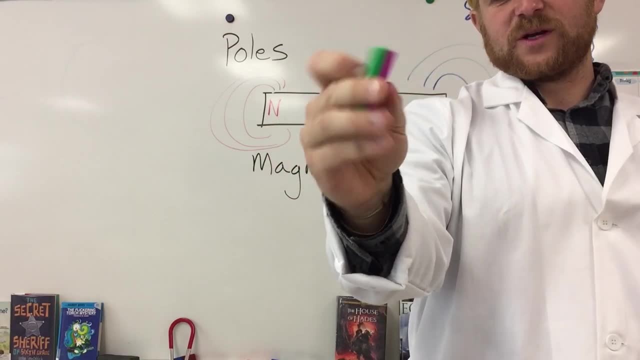 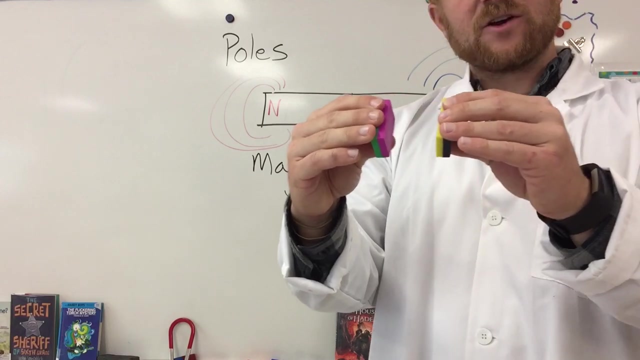 If I take these two magnets here, you can see this one's a green and purple magnet, with one of its fields green, one of them purple, and this one's a blue and yellow, And if I put them together you can see that these are the same field. It's either a north and a north or a south and a south. 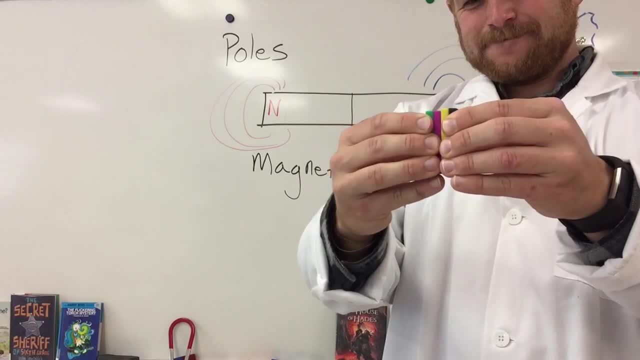 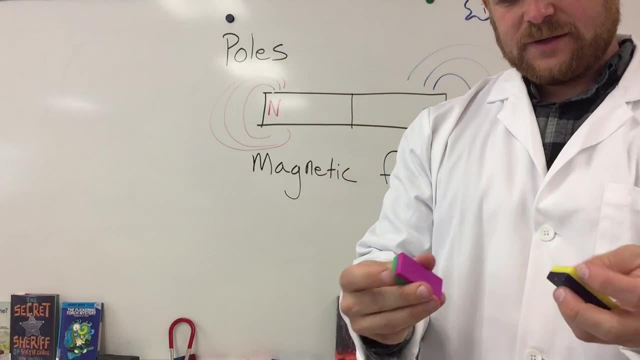 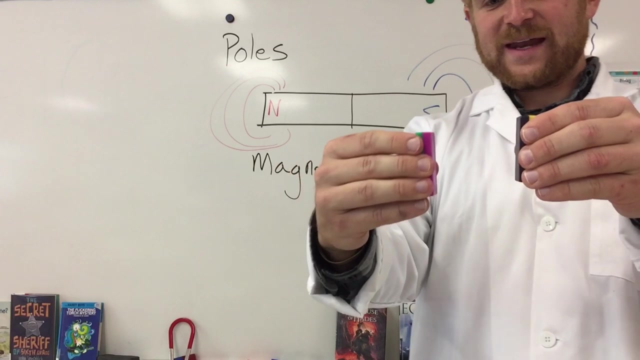 But there's no way to get them to hang out with each other. If I really squeeze them together, they'll actually pop it off. Now, if I put it together with the blue and the purple, these are opposing, So it must be a north and a south, and they really want to be together. 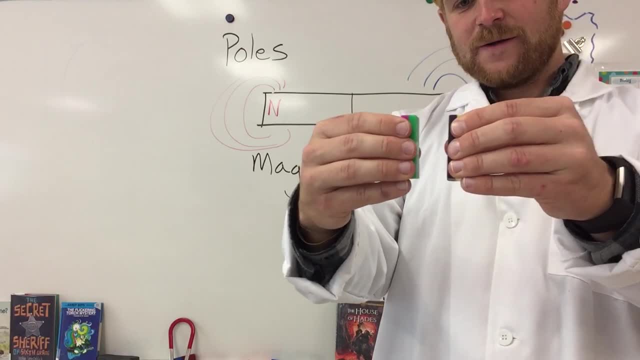 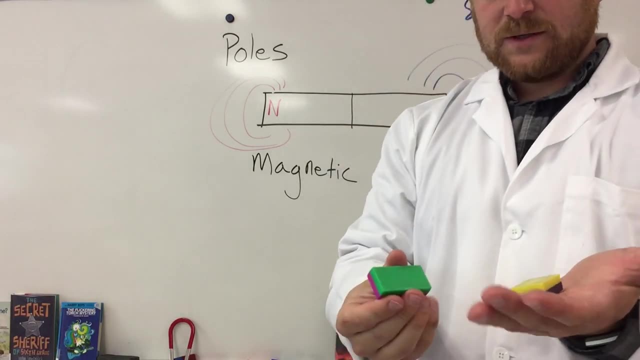 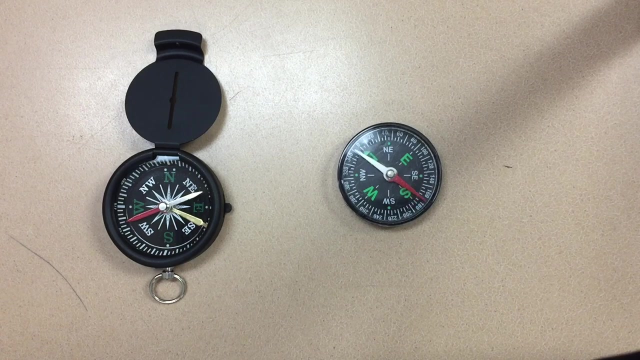 Where, if I flip it over now, it's the same pole and they won't stay together. Let's see if we can shoot it up one more time, Pew, And then I put them, and they stick. Magnets are found in all kinds of everyday objects. 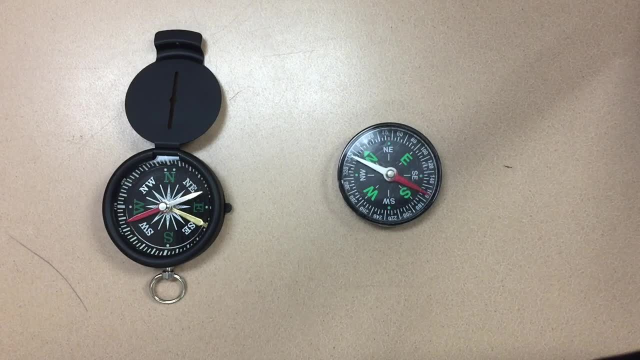 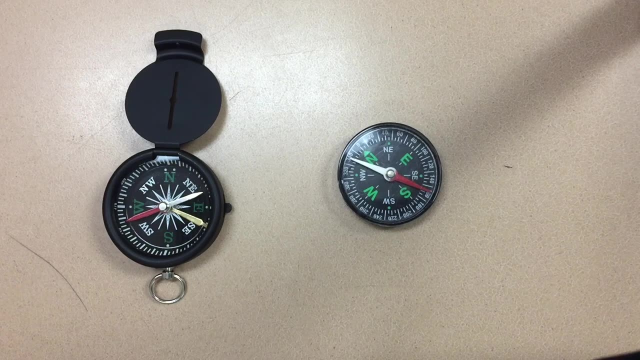 like these two compasses. These compasses use magnets to determine the north and south pole of the earth. Watch what happens if I introduce my own magnet to disrupt that field. You can see that it's got a North and a South pole. So if I put it in the fence, etc. and then you put it in the box, 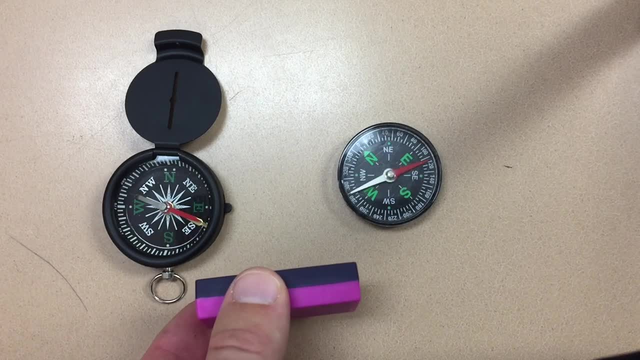 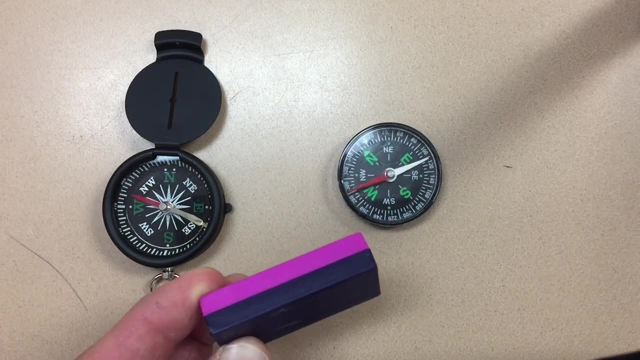 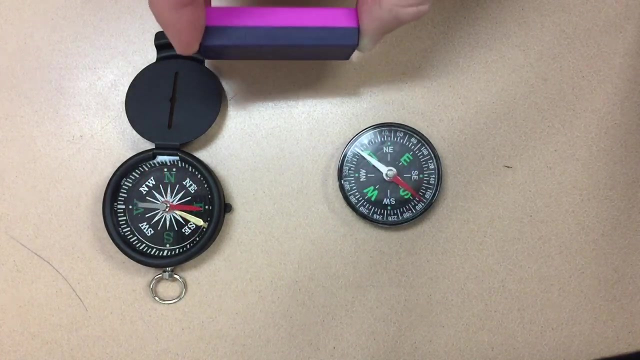 see, as I bring the magnet close, they're both attracted to my magnetic field. If I flip it, it'll flip them over and they'll be attracted to the opposite end. As I pull it through, they follow them. You can see that this magnet has a much stronger magnetic field than the Earth. 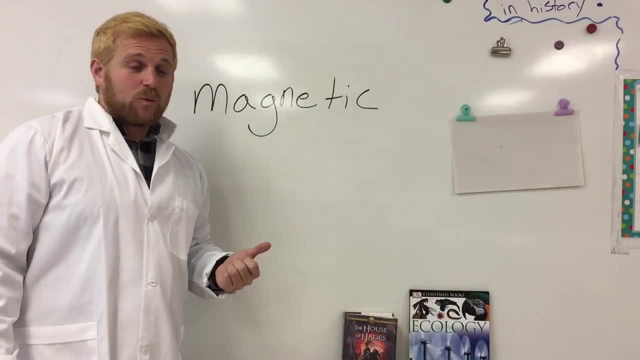 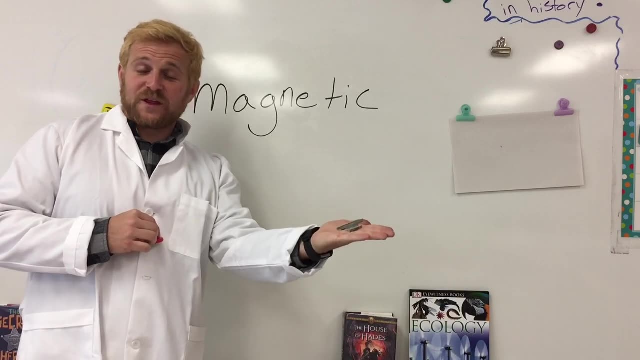 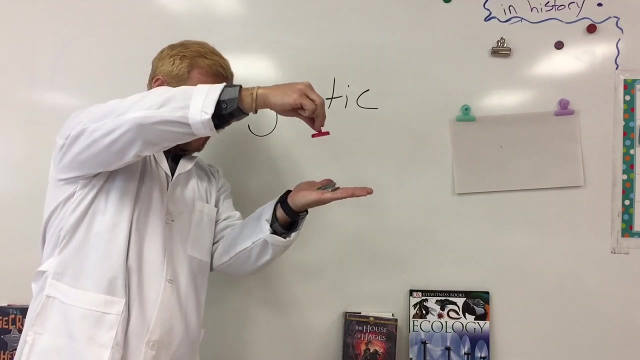 What do we mean when we say something is magnetic? We mean that it will attract or pull closer to a magnet. I have some staples in my hand. Do we think these are going to be magnetic? Let me hear you. All right, let's try it out. Look at that Magnetic. 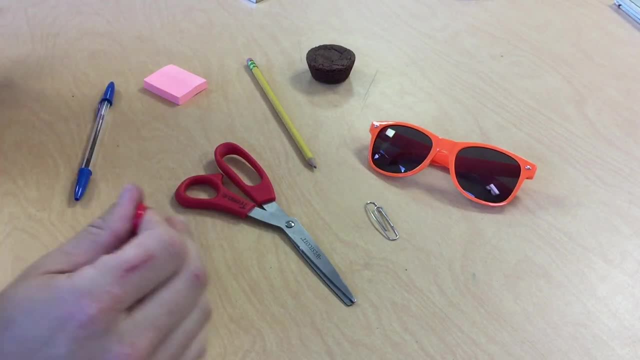 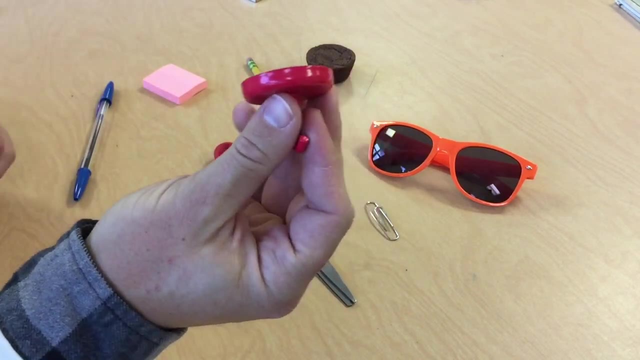 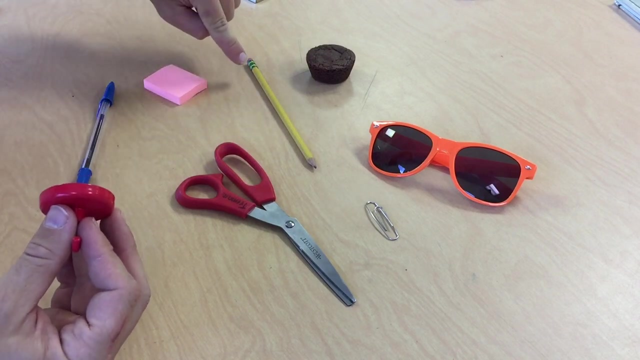 I laid some objects out on the table. Let's try and think which objects we think will be magnetic or will attract or repel to that magnetic field we talked about earlier. We have a brownie, some sunglasses, a paperclip, some metal scissors, a pencil. 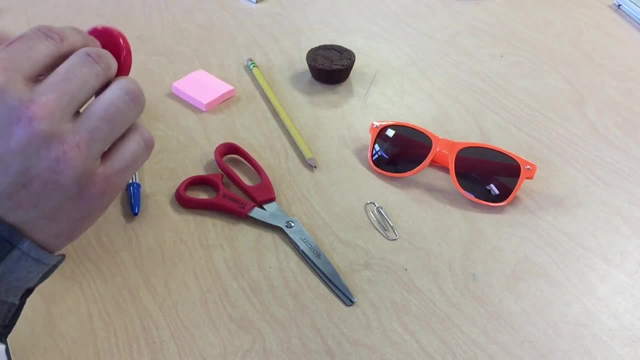 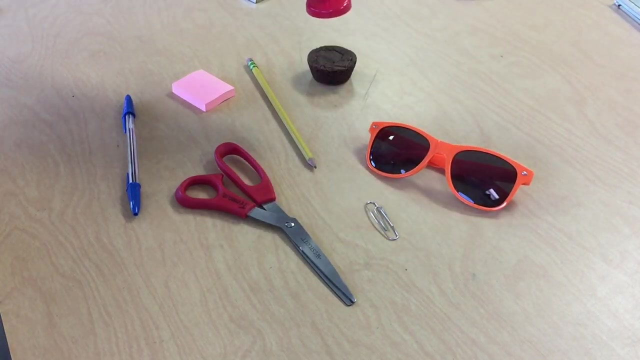 some post-it notes and a pen. Let's go around. Let's start with the brownie first. Do we think it's going to be magnetic? Nope, The brownie is not magnetic. Now, how about the sunglasses? The sunglasses are not magnetic. How about my paperclip? 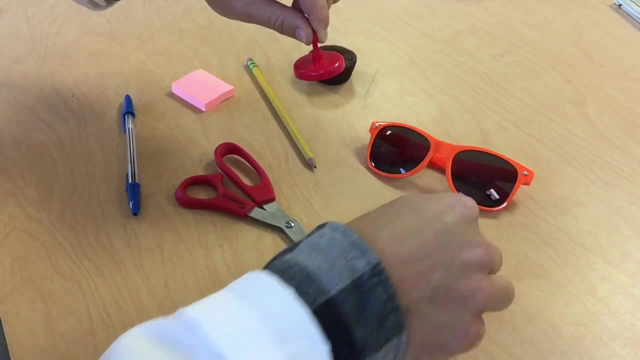 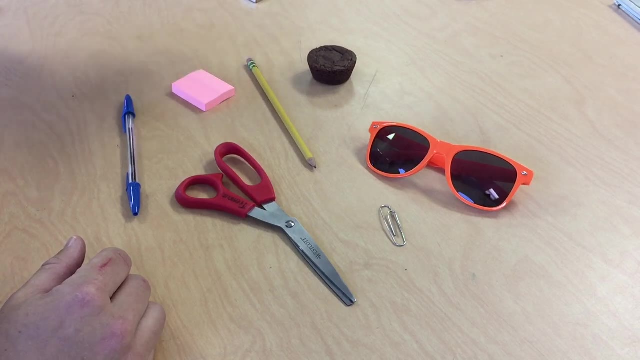 Wow, Did you see that The sunglasses are not magnetic? How about my paperclip? Wow, Did you see that My paperclip is definitely magnetic? How about the pencil? Nope, Not magnetic. Post-it notes- Not on my pen either. Let's try the scissors: Definitely magnetic. 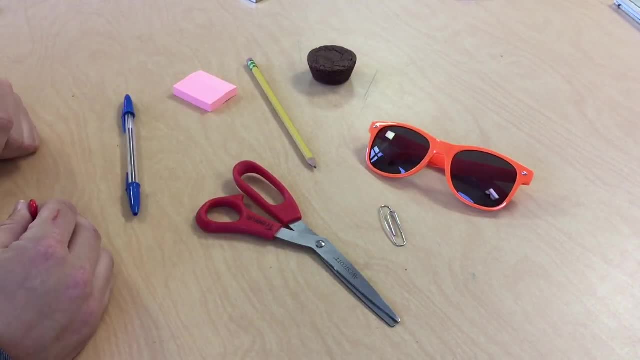 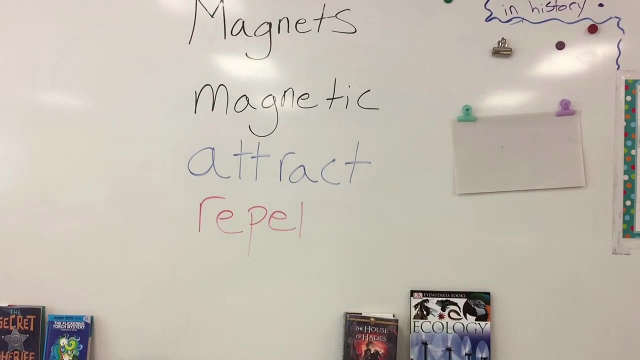 What do you think after looking at all these objects? What makes an object magnetic? My pen, my post-it note, my pencil, my brownie and my sunglasses were not magnetic. My scissors and my paperclip were. My scissors and my paperclip were.